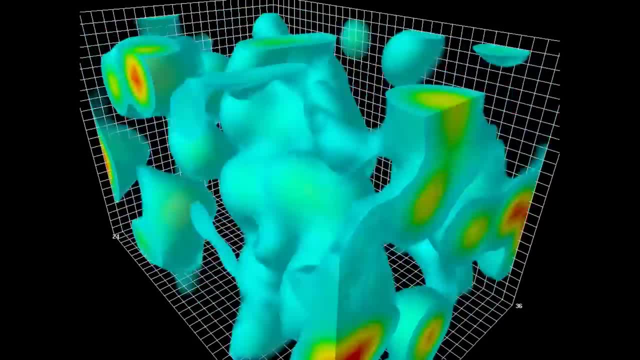 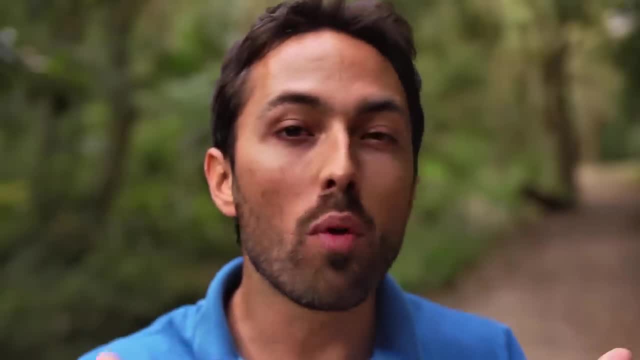 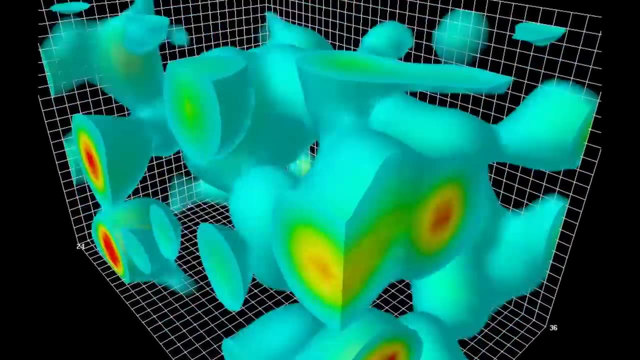 The dimensions of this box are absolutely tiny. They are millionths of a billionth of a meter. Roughly enough space to stick two protons, But there are no protons here. This is a simulation of the vacuum on its own, What we normally think of as empty space. 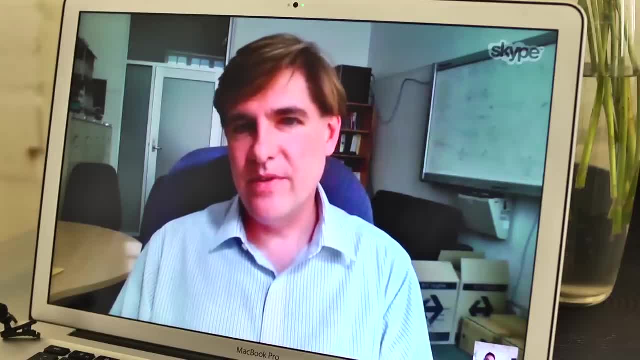 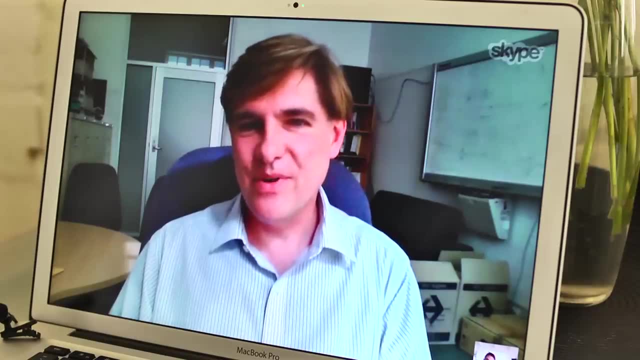 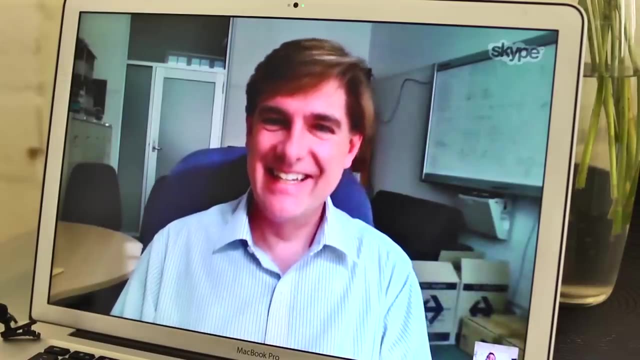 Empty space is actually full of these quark and gluon field fluctuations And on average it is possible to annihilate a quark from empty space because it's not empty. That just sounds like the most ridiculous idea: that you're meant to have empty space and yet you can go and get rid of stuff from it. 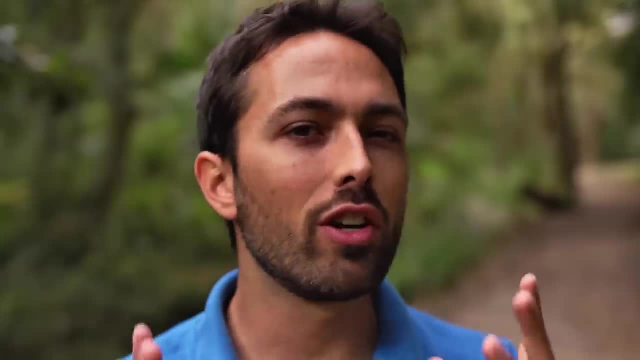 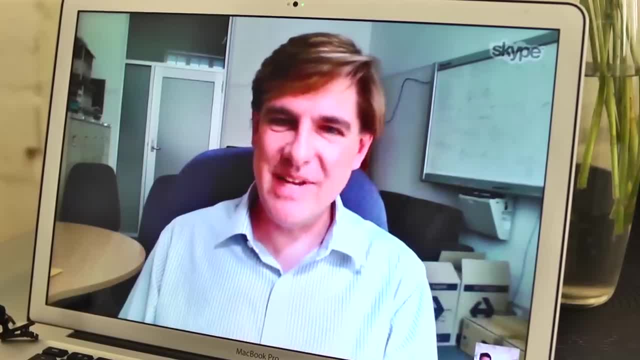 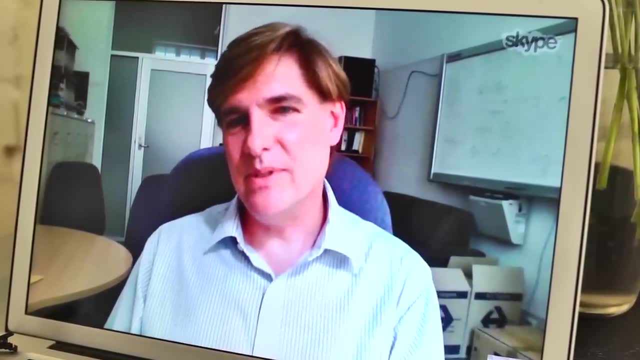 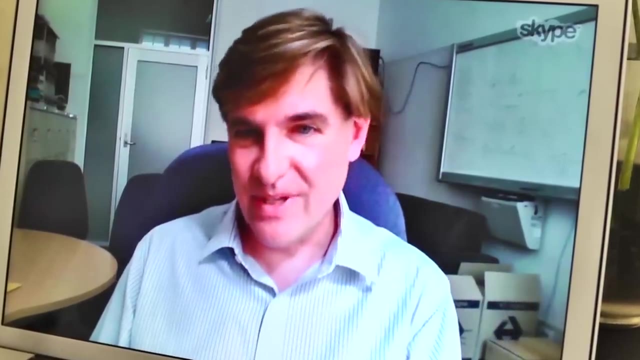 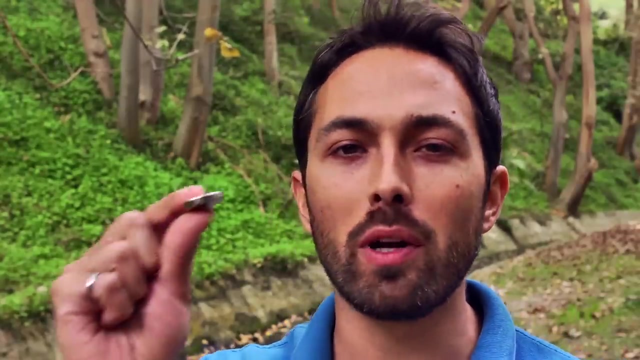 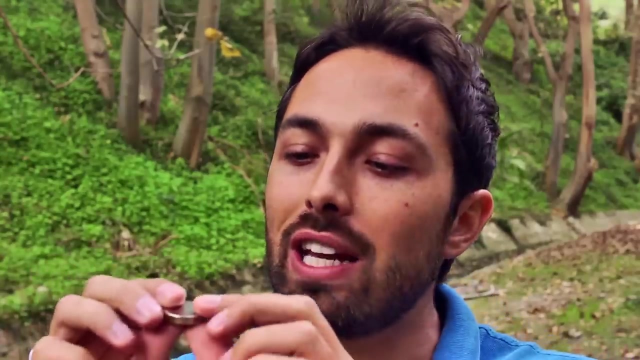 lot of energy. Well, this may not be as strange as it first appears. I mean, consider a permanent magnet. It has a magnetic field around it at low energy, at room temperature, and that's because the individual little magnetic moments of all the atoms inside are lined up. But if you were to heat it up you would give 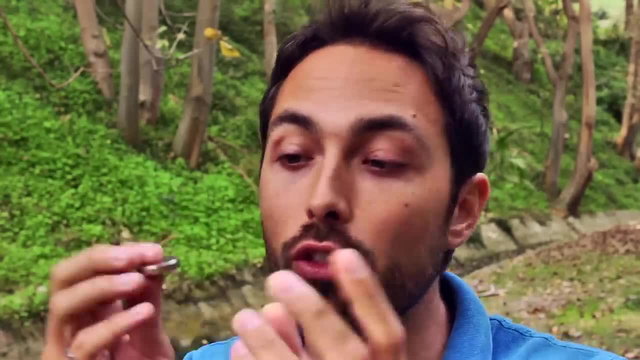 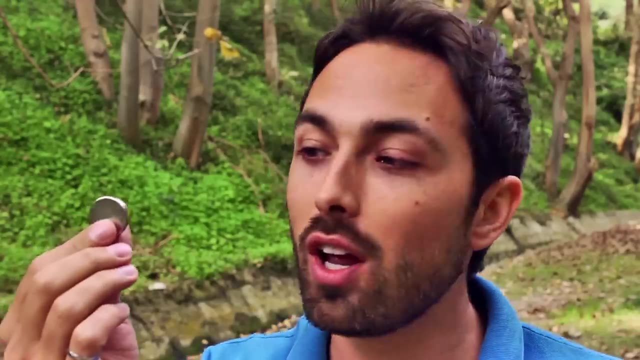 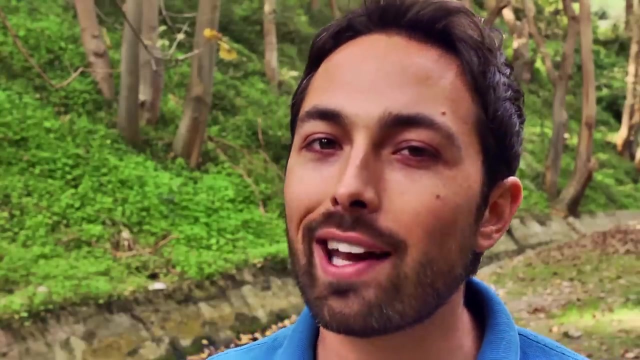 thermal energy to all those particles and at a certain point, called the Curie temperature, they would be so randomly aligned that there would no longer be an overall magnetic field. So it actually takes energy to get rid of the permanent magnetic field. This is just like the quantum vacuum and understanding how the 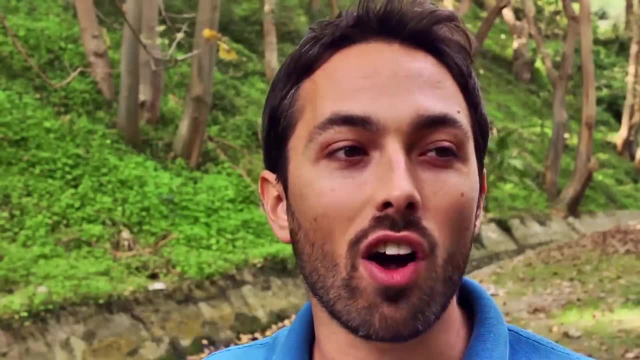 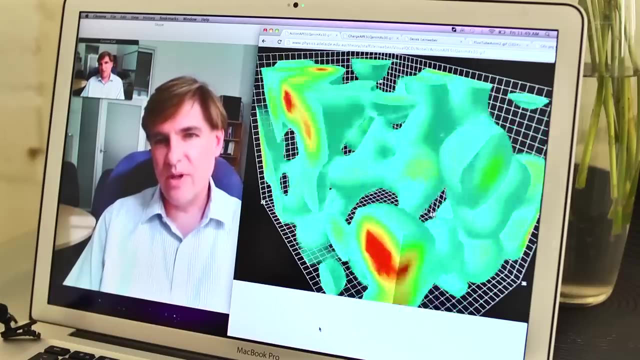 quantum vacuum fluctuations work gives us a sense of what the fundamental particles do like. where are you most likely to find a quark? And it turns out that the quark likes to sit on top of those lumps. Now those lumps come into and out of.